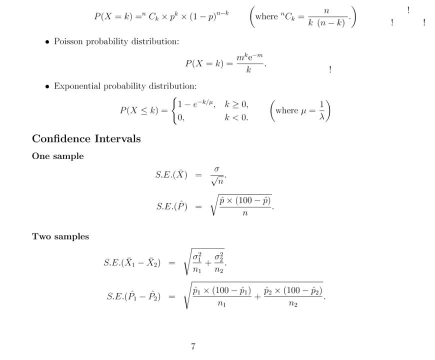 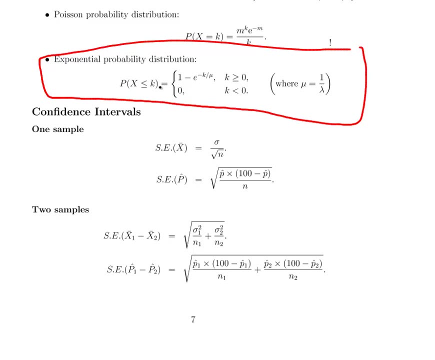 So I'll just go through the exam paper there And we'll pick this out. This is what we're looking for. Okay. Now the probability of x less than or equal to k is equal to 1 minus e, to the minus k over mu. Okay, So I'll write that out again. By the way, k has to be greater. 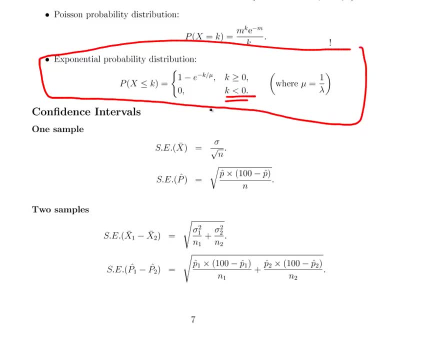 than positive. Well, it actually has to be known as zero to be correct, So we're going to have a slightly simplified version of that. Sometimes, actually, the question might be posed in terms of the rate parameter lambda, where the mean is just the inverse of the. 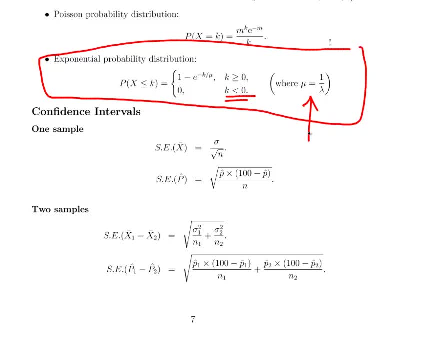 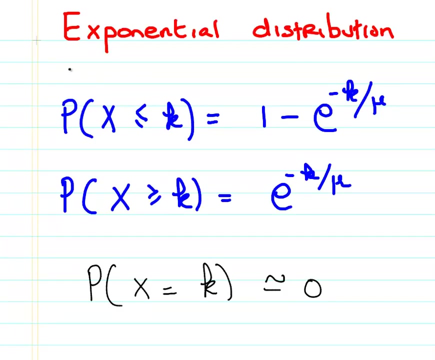 rate. So it's just watch out for that. So I'm posing the question here in terms of the exponential mean, But some other questions might sort of give you the rate instead. So it's just one times the one over the mean, Okay. So let's get started here. So this is: 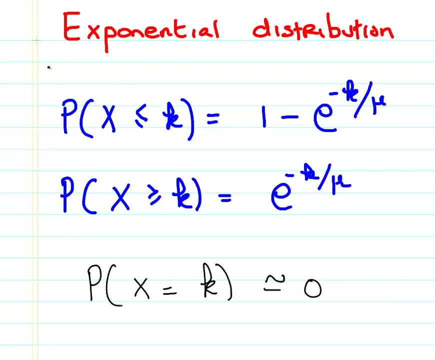 the formula, And this is a sort of reduced version of it, because we'll work on the basis that x is greater than or equal to zero, Okay, so, So this is the main formula we're given: Okay, Where k is some constant. okay, x is the lifetime, k is some constant and mu is. 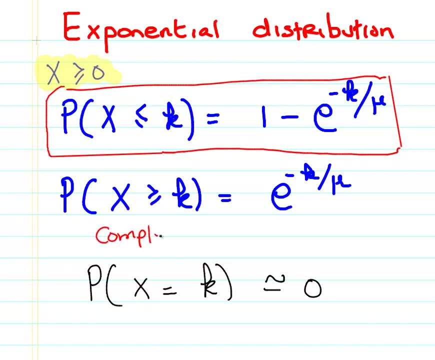 the mean. Now, this here is the complement: probability. It's a complement of that formula. It's a little bit simpler: e to the minus k over mu. Okay Now, so essentially, just as a remark, I get asked this all the time: is that the complement? How do you know this? 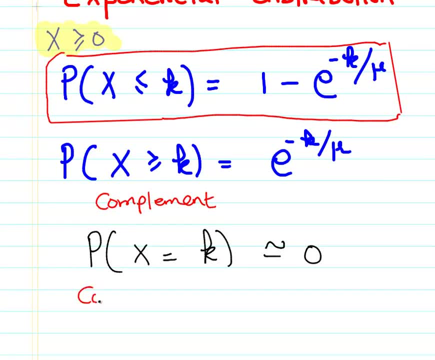 How does that make sense? Essentially the probability, but this is the thing for continuous random variables. the probability of x taking a very precise value or a value very precisely, is considered to be negligible to the extent that it's impossible, It's zero. Okay, So that's how we can write the complement of this as this: Okay, So it's. 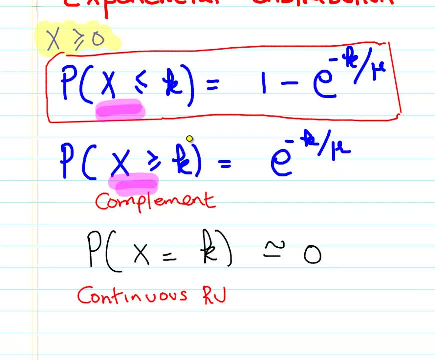 a little bit of a cheat, but it actually works fine mathematically Okay, If the probability of x equal to k is considered to be zero, which is the case for continuous random variables. Okay, So let's just get started on this. The first one is probability of x being less than. 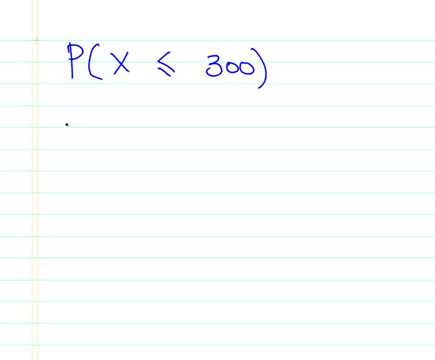 300, as in that the component fails within the first 300 hours. So that is 1 minus the exponential of minus 300 over 1200.. That is 1 minus e to the minus 1, 0.25.. Okay, So on your calculator what you should be pressing there is the exponential. 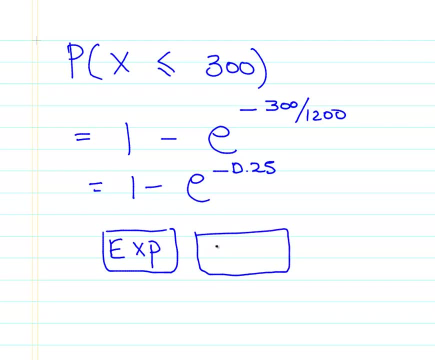 That's one of the buttons on your calculator, and then just type in minus 0.25 in brackets, or something like that. That's what you do with your calculator, calculator, and then subtract that from 1.. So let's just calculate that out. 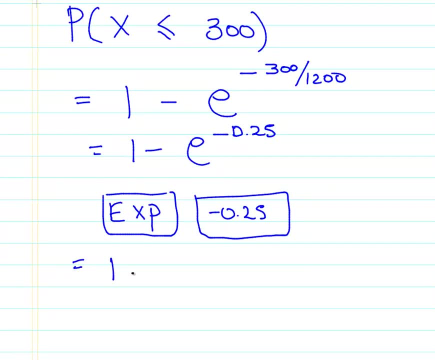 That is equal to 1 minus 0.7788, roughly So that is 0.2212.. So that's their answer. The 22% approximately of components will fail within the first 300 hours. Seems like a lot, doesn't it? 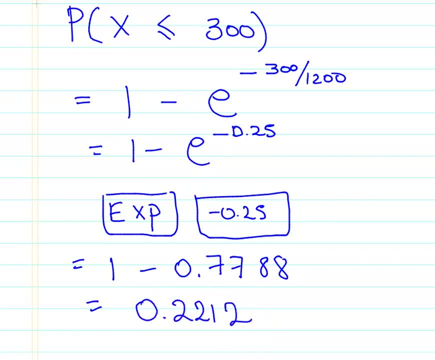 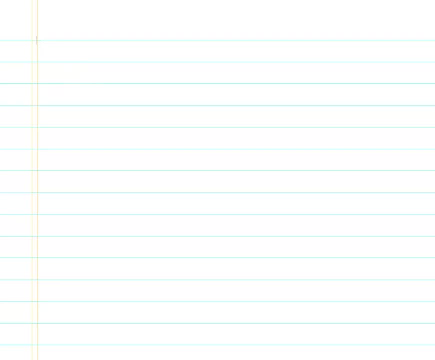 But there you go. So that's the first answer to the first one. The second one is the probability of lasting more than 1,500 hours. So the probability of lasting more than 1,500 hours, that is, e to the minus 1,500.. 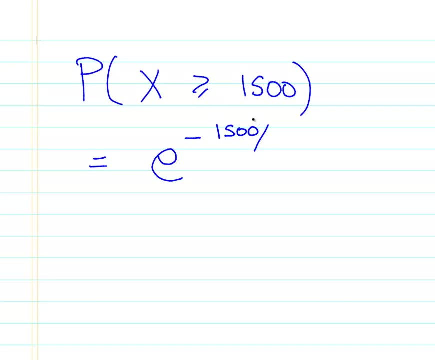 Sorry, that's 1,500.. Sorry, 1,500.. 1,500 is 1,500, just in case you're not familiar with that sort of use of the phrase. This is again a little bit of calculator work. 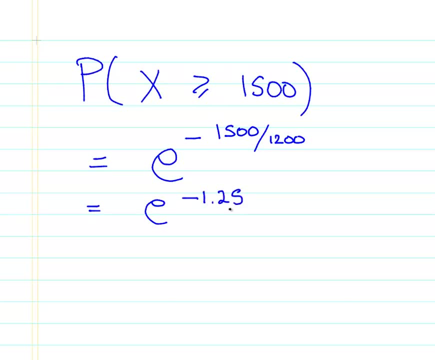 e to the minus 1.25.. And again it works out the same way as it did the last time with the calculator. Just we should get 0.2865.. That's the answer to the second one. And finally, this one's a. 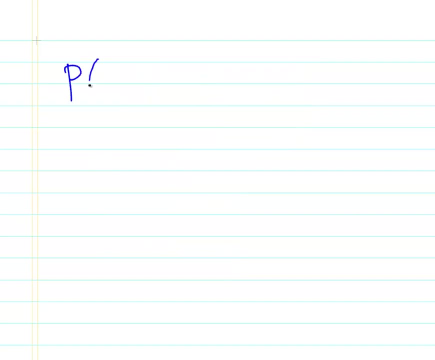 little bit longer: The probability of lasting between 1,200 hours and 1,500 hours. So what we have here is an interval, And the probability of being inside that interval is the complement of the probability of lasting between 1,200 and 1,500 hours. 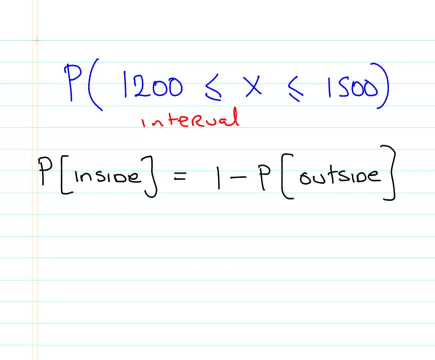 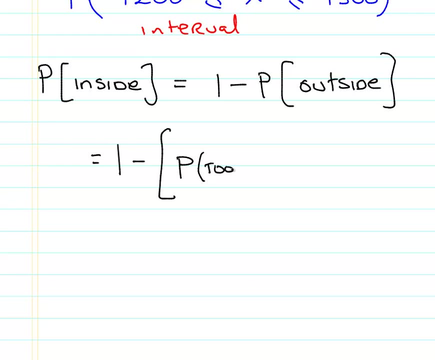 So that's the probability of being outside that interval, And the probability of being outside that interval is being the combination of probability of being too low plus the probability of being too high. Okay, So we can break the problem down to two very simple subproblems. 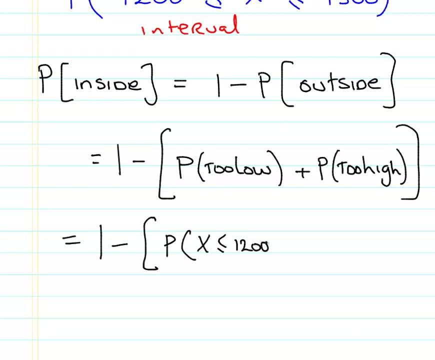 So this is the probability of x less than or equal to 2.. And this is the probability of x less than or equal to 2.. or equal to 1,200 hours, And this is the probability of X being greater than 1,500 hours, which. 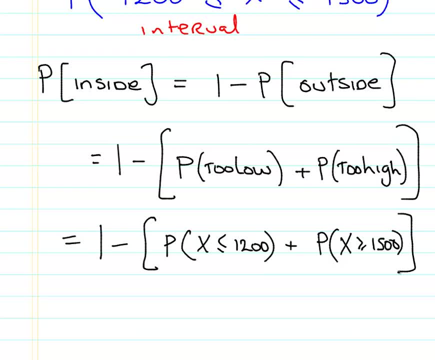 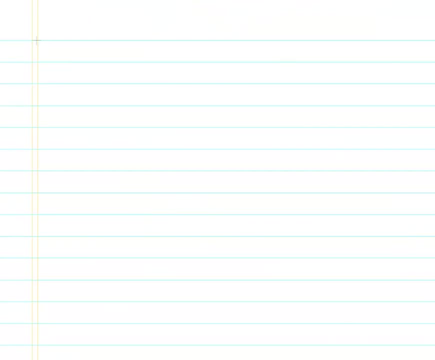 is one we just calculated already, So we don't actually need to do that again. Okay, So the probability of X being less than 1,200.. Now, remember, that's the mean. You're going to find this answer a little bit strange, But you know, just bear with me in this, That's. 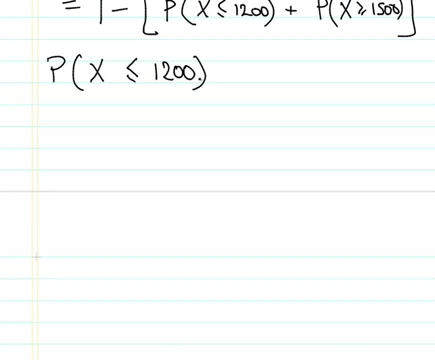 the average. Well, not as intuitive as you think, But remember this is a skewed distribution. So this is 1 minus the exponential of minus 1,200 over 1,200.. Okay, And that is not point 6,321.. Okay, So that's the probability of being too low as in the lifetime is less. 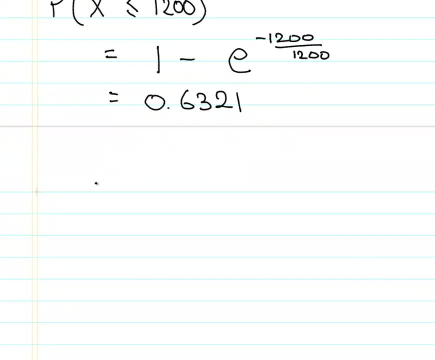 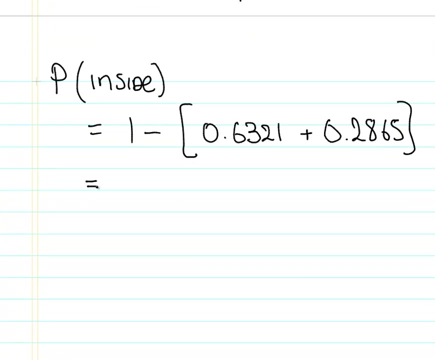 than or equal to 1,200.. So let's just piece it all together. So the probability of being inside our interval is 1 minus, not point 6,321.. Okay, Plus, not point 2865.. Okay, Little bit of calculator work. I made that to be about. 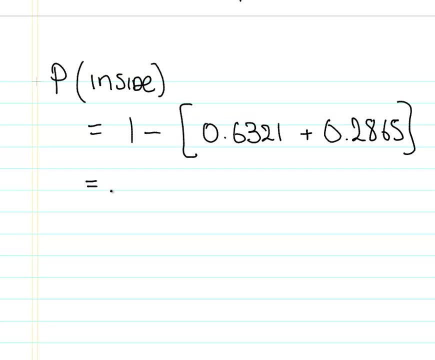 91% approximately. Actually just want to sort of give you the final answer here, allowing for a little bit of rounding error, because I'm just reading this off some computer output. That is my answer there for the last one. Okay, So that is an exponential distribution. worked example. Okay.